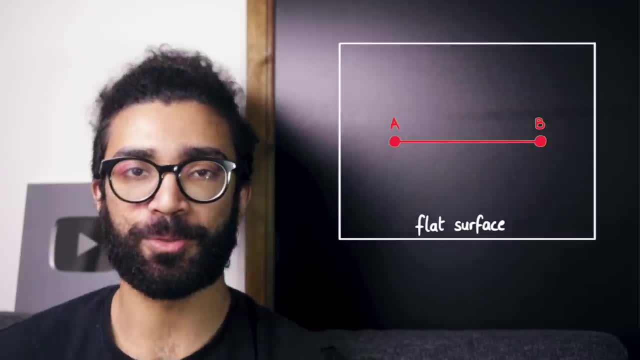 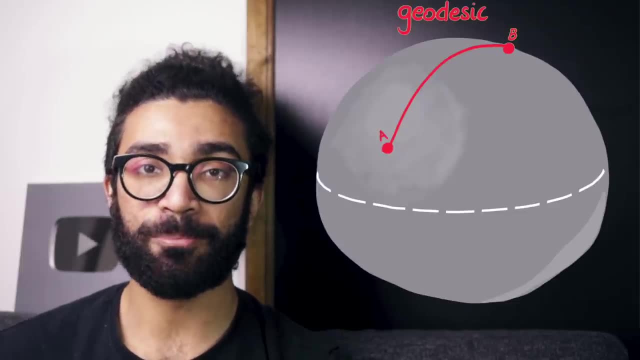 and technically, the path that we saw earlier on a flat surface between points A and B, the straight line path, is also a geodesic. But if we continue to think about our spherical surface with points A and B on this sphere, the geodesic between any two, 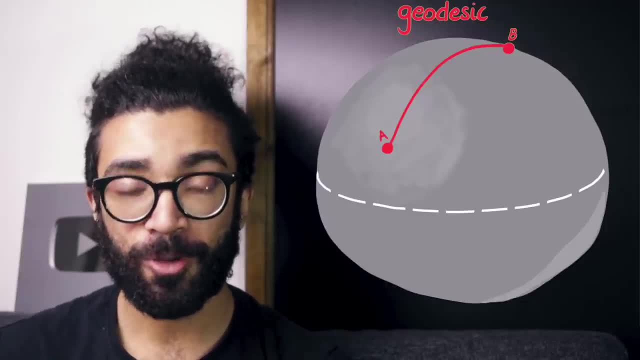 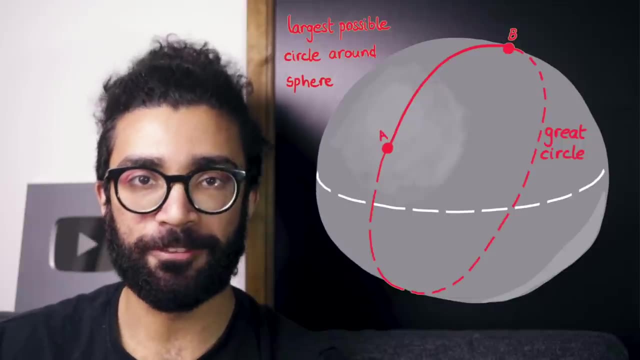 points, say, points A and B- is always going to be a section of what is known as a great circle. A great circle is simply one that is the largest that you can create for any given sphere. It's essentially the diameter of the sphere- Another way to think. 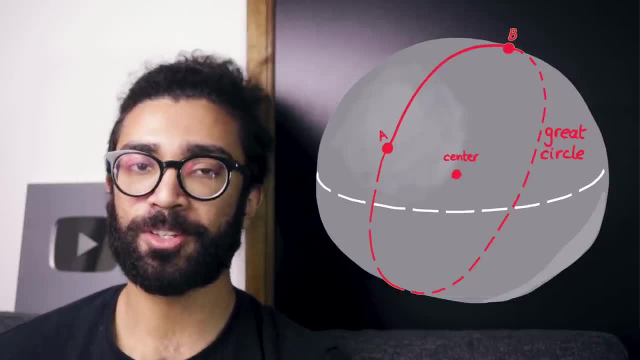 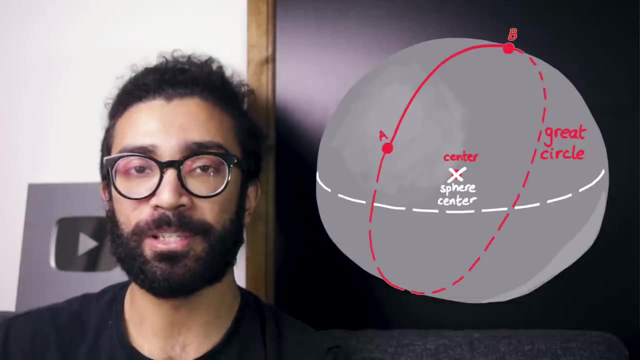 about this is that the center of a great circle is also the center of the sphere that we happen to be considering. As an easy way to remember this, if the surface that we happen to be considering happens to be the surface of the earth, then the equator would be a great circle. 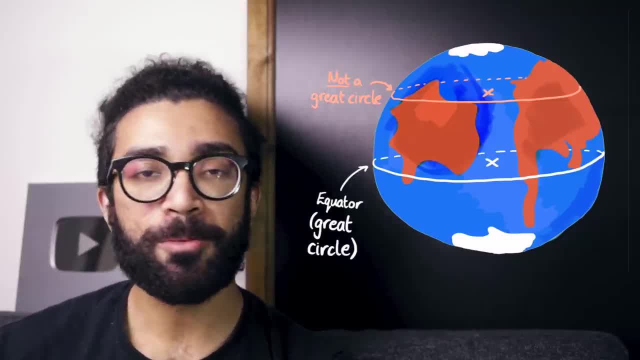 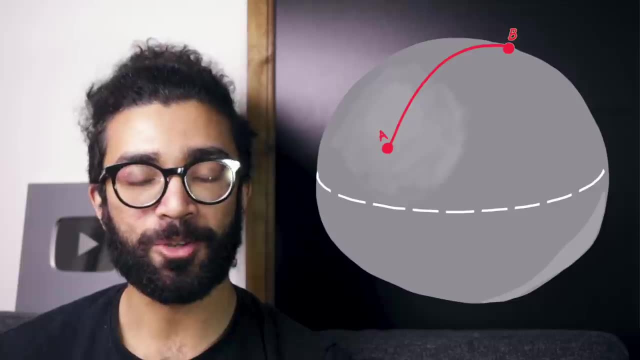 but any of the other lines of latitude would not. So, coming back to the point we made earlier, if there are two points on the surface of a sphere, the shortest distance between them along that surface is always going to be a part of a great circle, For example, 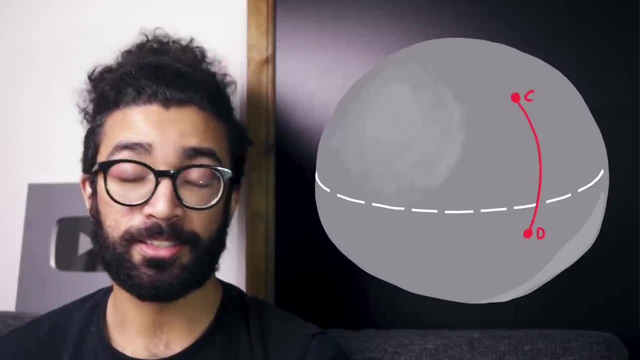 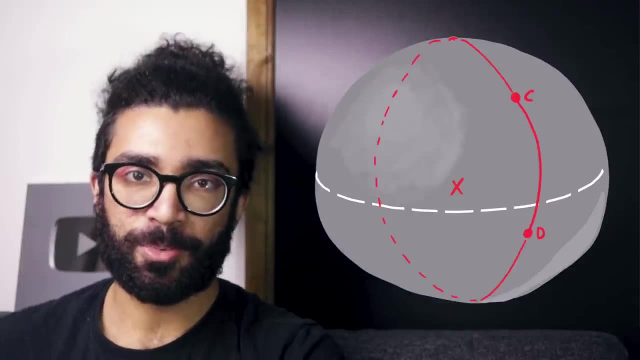 if we choose another two points, C and D, the shortest distance is this one here, and that is a part of another great circle. Now, this is all well and good, but the reason that the shortest distance between two points in a sphere is not a straight line is because we restricted. 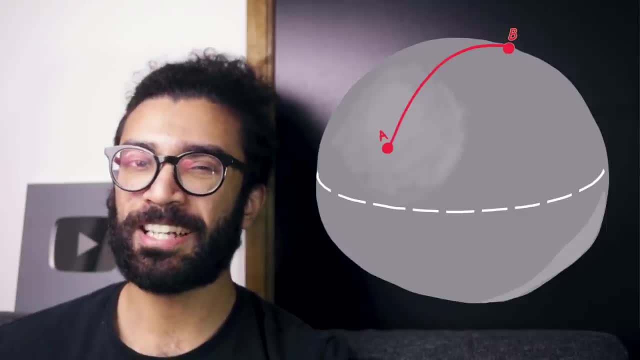 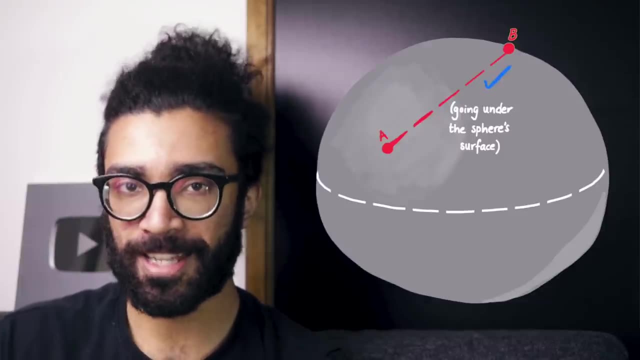 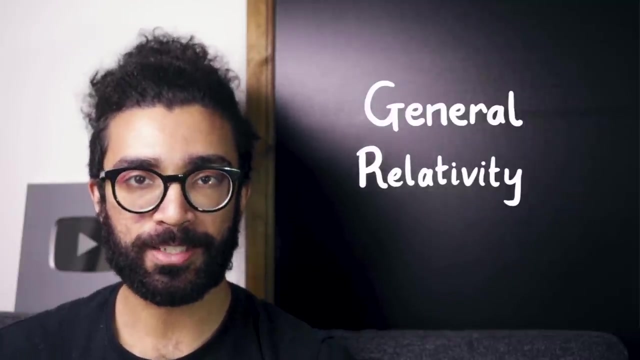 it along the surface of the sphere. But if that restriction did not hold, then technically the shortest distance is still the straight line distance between those two points. This kind of logic unfortunately breaks down a little bit when we start studying general relativity. Now, in the study of relativity we often consider what is known as the shortest interval between: 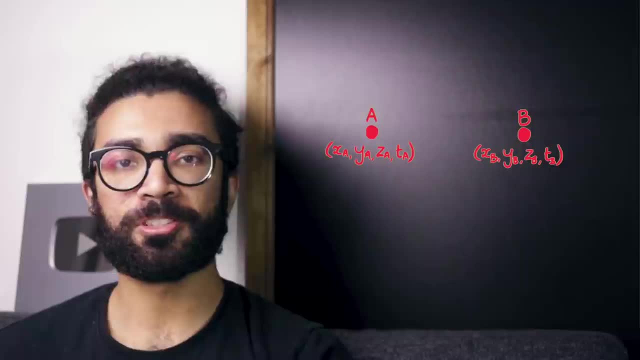 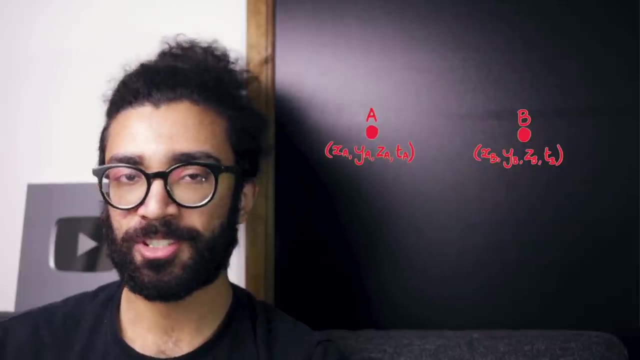 two events. This is essentially just a four-dimensional space-time version of what we were just talking about: the shortest distance between two points. The logic is essentially the same, just extended up to four dimensions, And the reason that we do this is because, in relativity, 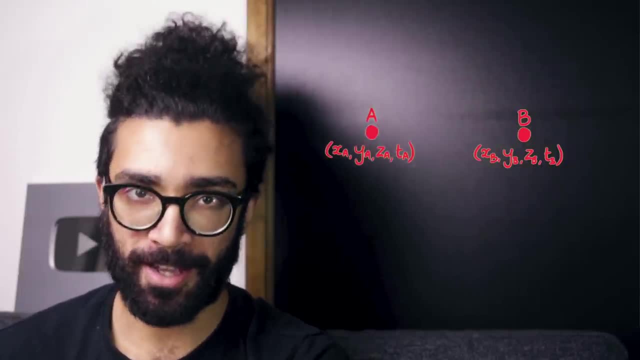 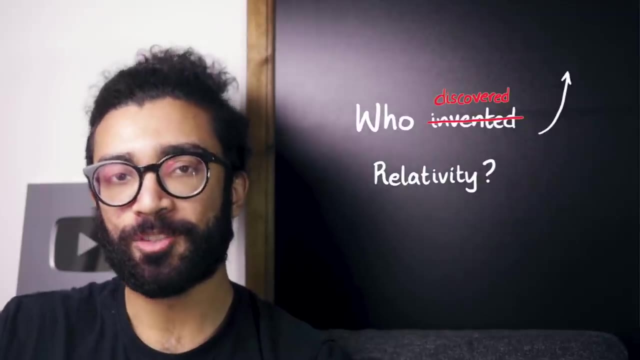 we study the three dimensions of space and the fourth dimension of time. By the way, if you want to find out more about four-dimensional space-time, then check out this video I made a little while ago on my channel. Now, one of the reasons we study the shortest interval between two events in general, 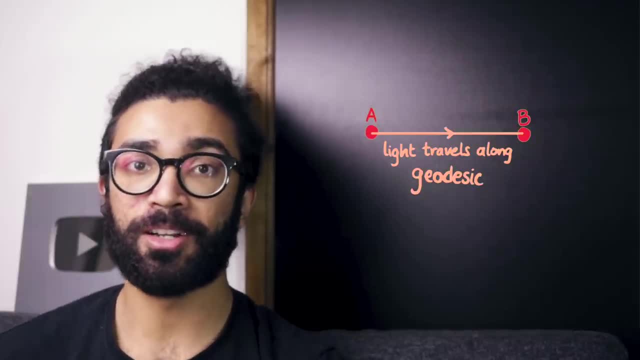 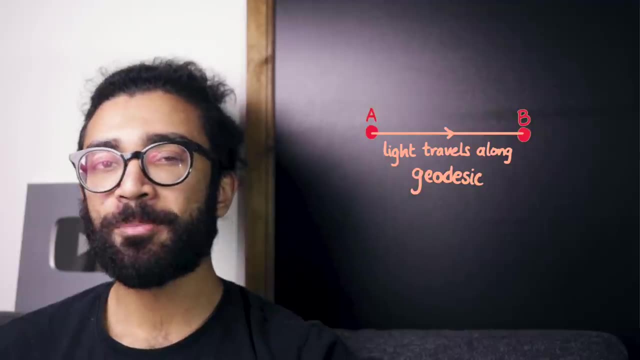 relativity is because light travels along this kind of geodesic, And an important aspect of general relativity is how light travels through our universe. Let's now imagine that we're thinking about two events in empty space-time. Other than these two events, there's basically nothing around. 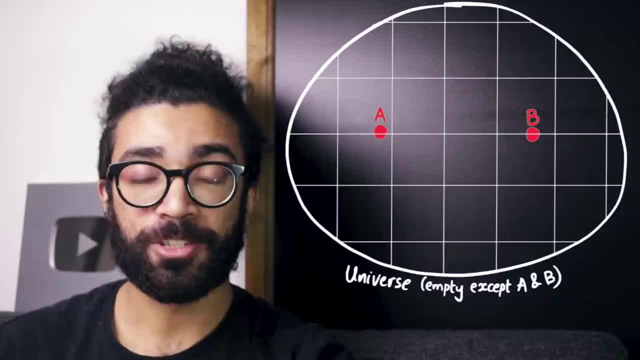 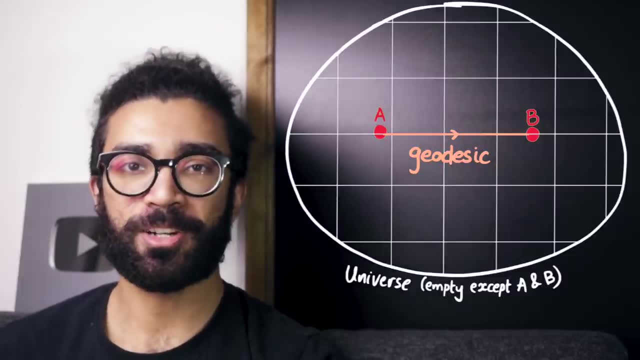 no stars, no galaxies, no nothing. Well, in this situation, our geodesic- the shortest interval between these two events- looks kind of like our straight line example from earlier. Remember, though, that this illustration is a two-dimensional representation of 4D space-time. 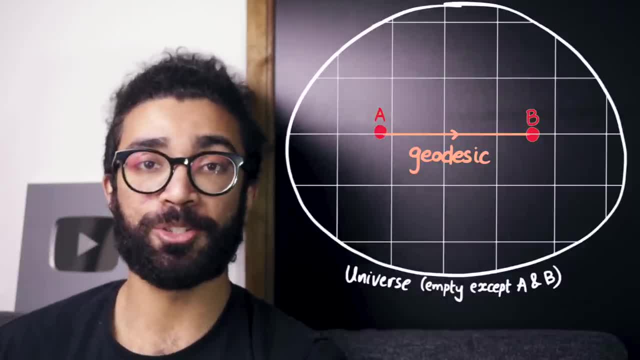 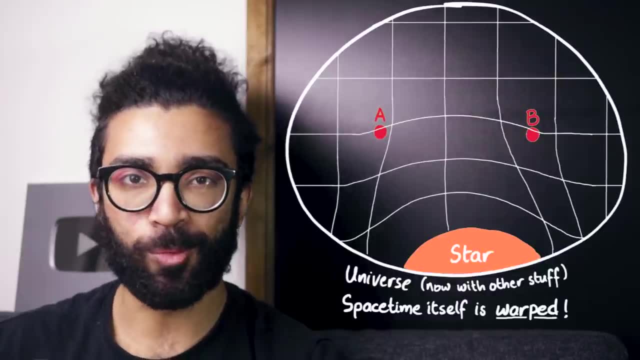 so it's kind of cutting some corners and so on, but it's a good visual tool Anyway. so dealing with this kind of space-time- empty space-time- is pretty simple. But what happens when space-time is actually warped? According to Einstein's field equations, any amount of mass or energy within 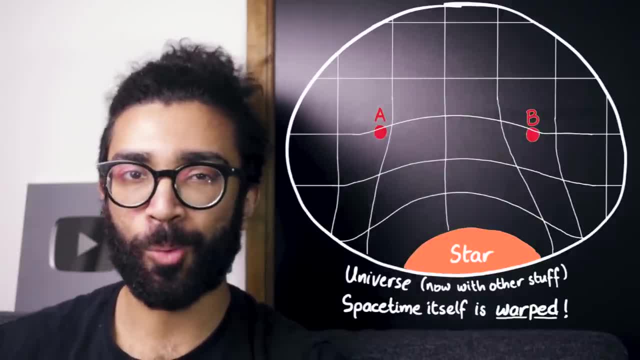 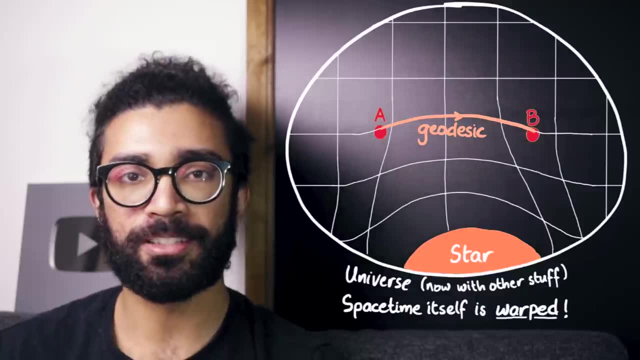 a region of space-time causes the space-time around it to warp or bend, And this will inevitably affect the shape of our geodesic, because the idea of an interval between two events in space-time only really makes sense if we think about it as being part of our universe or our space-time. 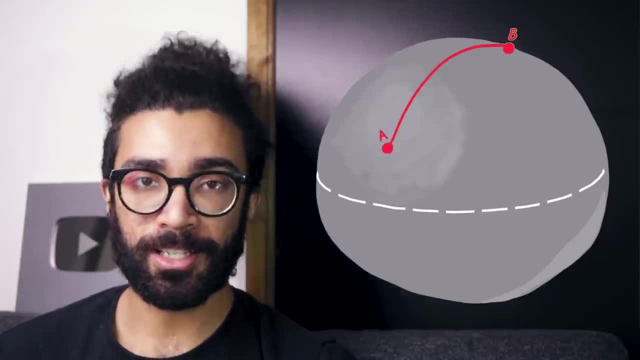 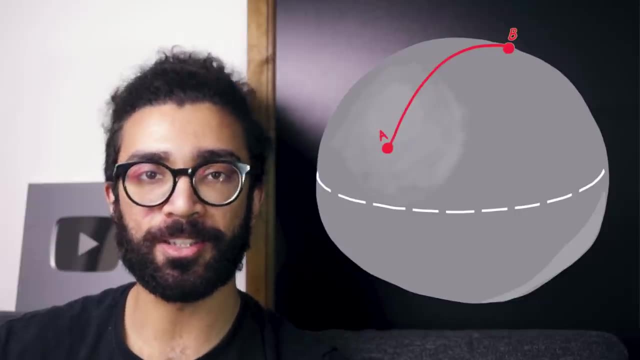 So this scenario is slightly different to the sphere example from earlier. In that example the shortest distance between a and b was our curved geodesic, if we were restricted to being on the surface of the sphere. But in reality the actual shortest distance between the two points was the straight line between a and b. 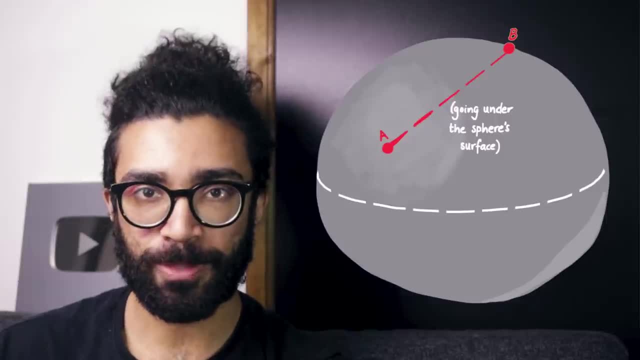 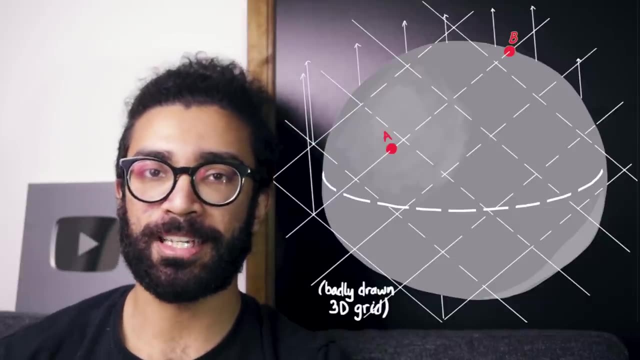 The problem with this depiction, though, is that it implicitly assumes that our sphere is somehow located in some three-dimensional space. This is the kind of space that we experience on a day-to-day basis, that we assume exists around us, And this idea where our two-dimensional 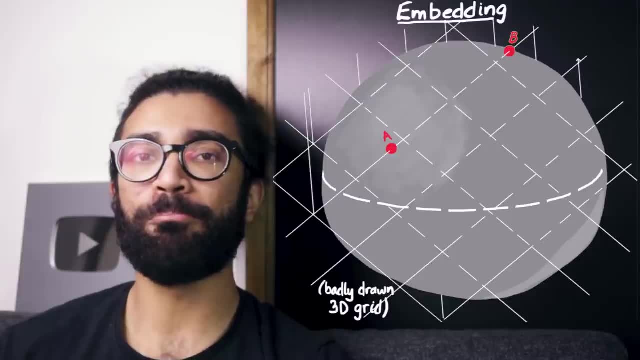 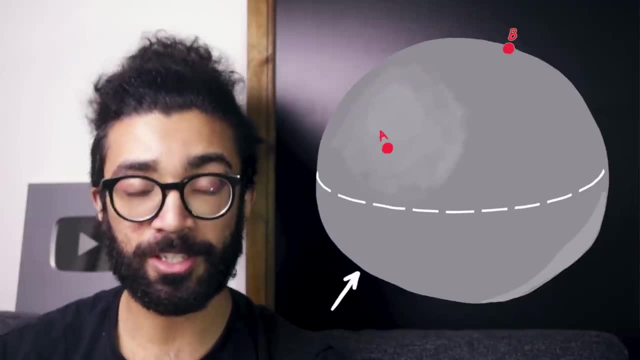 sphere is located inside a three-dimensional space is known as embedding in relative relativity. We use embedding in order to help us visualize what's going on with, essentially, a curved surface, a curved two-dimensional surface, but relativity tells us that embedding is not. 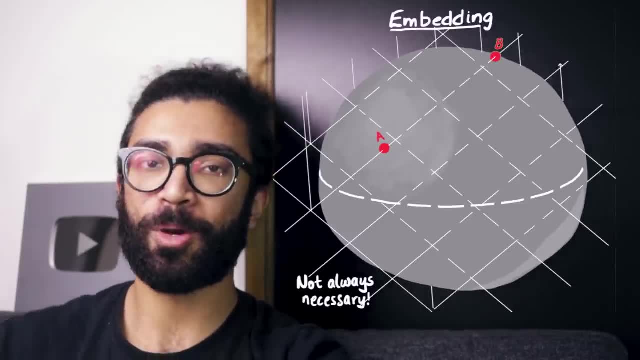 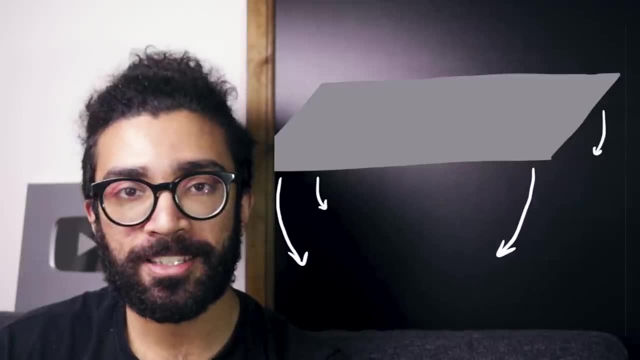 always necessary, And we could just choose to consider a surface where going into the sphere doesn't really make any physical sense. To clarify, this is a two-dimensional surface that is warped into the shape of a sphere, and so it only makes sense to go along this surface, And so. 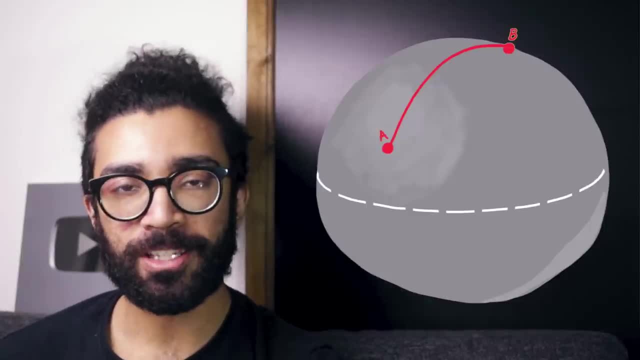 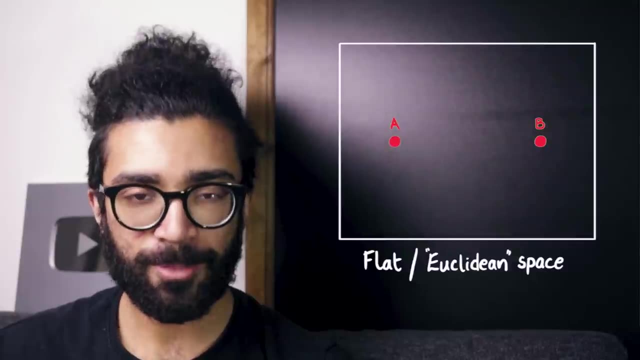 the shortest distance between two points on our surface need not be a straight line. That is only true in flat or Euclidean space. Not convinced by this argument, Well, let's imagine that our surface, our sphere, is a plastic ball embedded in some three-dimensional space. So it's. 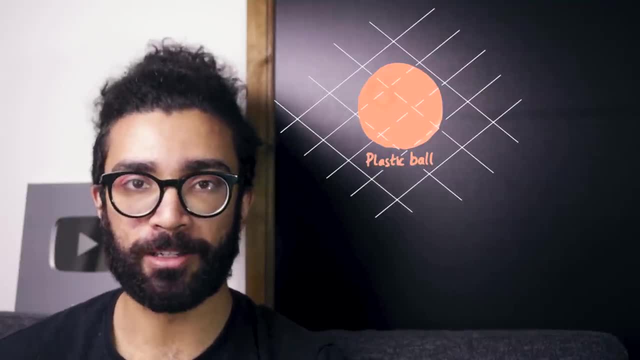 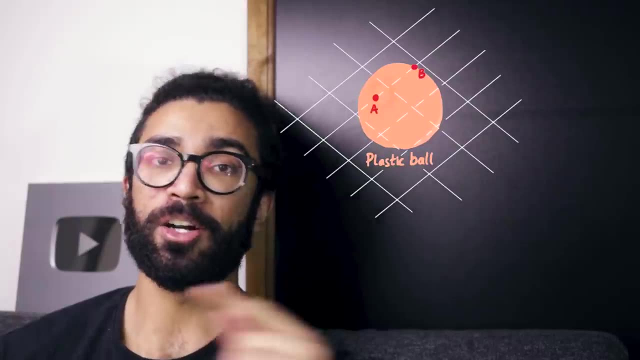 just a plastic ball existing in our universe as we experience it on a day-to-day basis. And so if we imagine two points on our sphere, then the restricted shortest distance between them is our curved geodesic, but the actual shortest distance is this straight line. 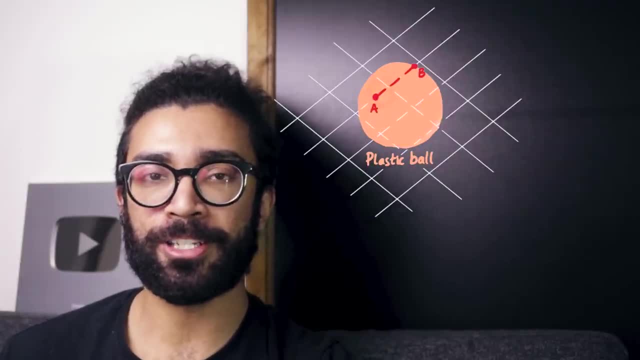 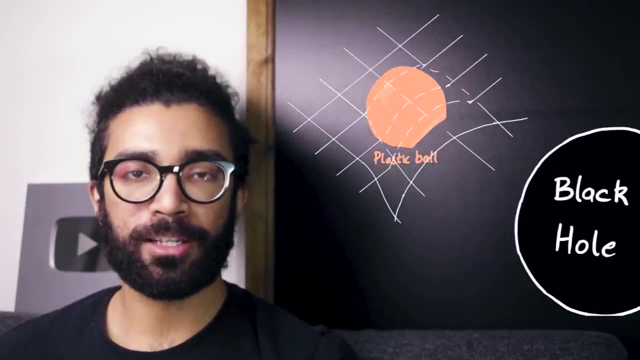 But what if we now take this plastic sphere and place it somewhere in a region of warped spacetime, Maybe somewhere close to like a black hole, for example? Say, it's not near enough to fall into the event horizon, but it is near enough to experience the 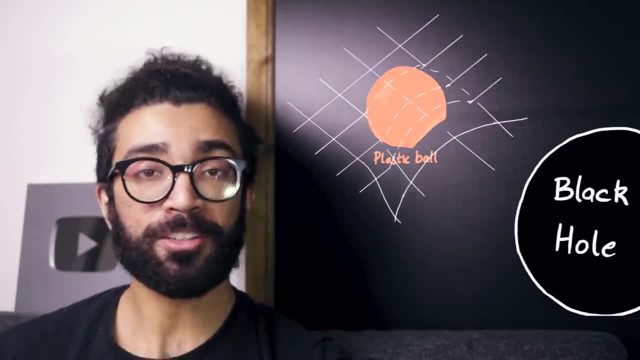 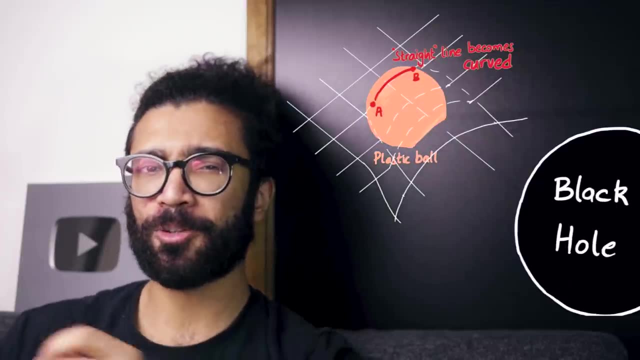 spacetime warping effects of the black hole. Well, in this scenario, because spacetime is warped, even what we think as the actual shortest distance between points A and B is itself going to be a curve. because spacetime itself is curved, The straight line between points A and B has no 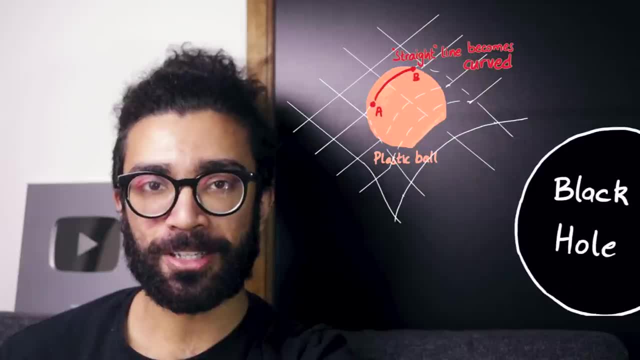 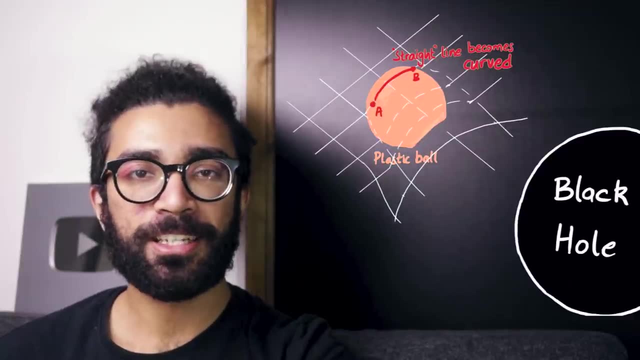 physical meaning at all. This is a rather tricky idea to get your head around, and in order to convince yourself of this, you'd have to study the general relativity mathematics in a bit more detail. The explanation I've just given is a way of visualizing it without all the gory mathematics. 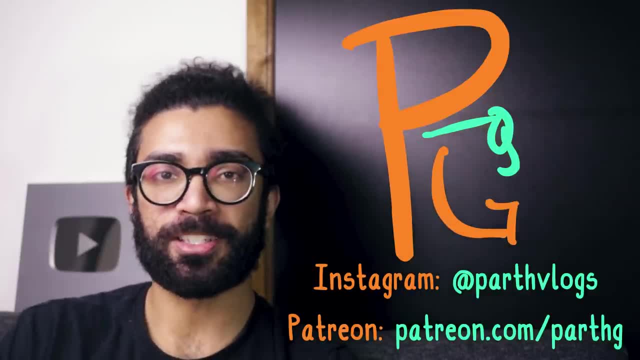 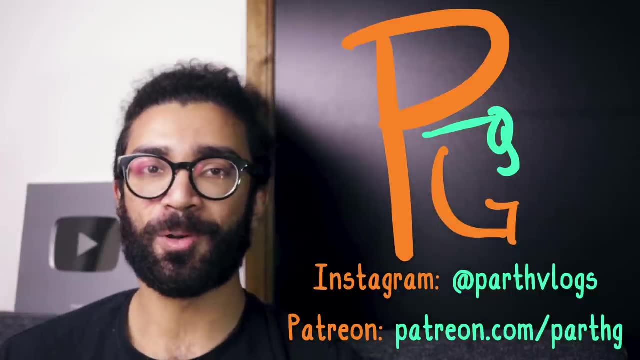 but don't take my word for it. Learn general relativity. It's super interesting. I'll leave a link to a textbook that I used when I was studying at university down in the description below, But of course, you can learn it literally anywhere. at this point, There are lots of different. 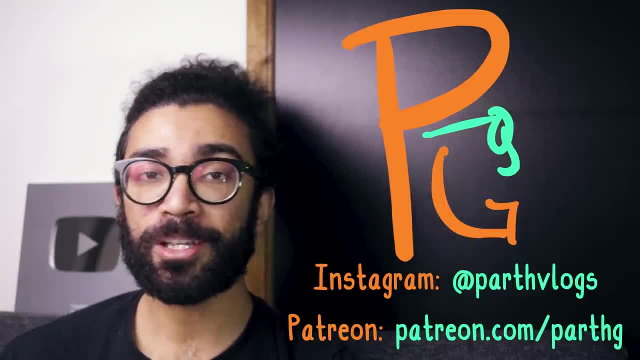 videos on it on YouTube, going through the maths in more detail, and even Wikipedia is a useful resource. And with all of that being said, I'm going to finish up here. Thank you so much for watching. If you enjoyed this video, please give it a thumbs up and don't forget to subscribe to. 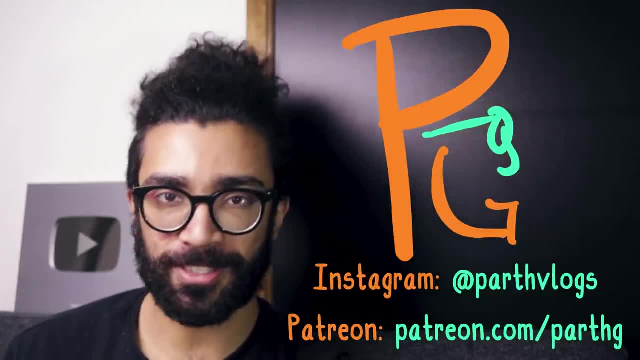 my YouTube channel. I'll see you in the next one. Bye. If you enjoyed this video, then please do hit the thumbs up button and subscribe for more fun physics content. Hit that bell button if you'd like to be notified when I upload. 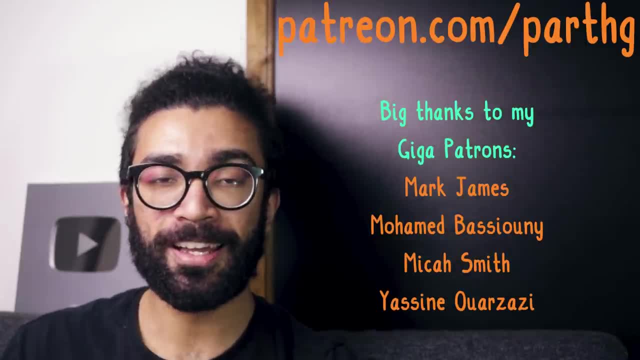 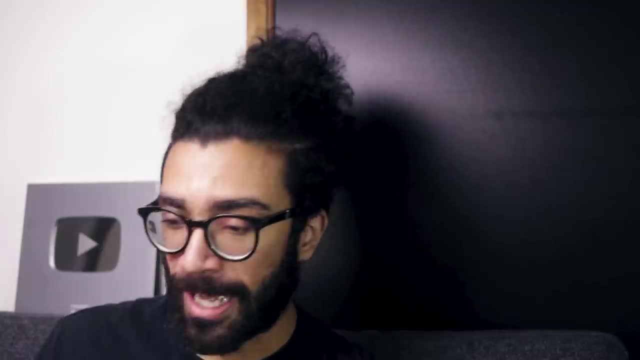 and please do check out my Patreon page if you'd like to support me on there. Thank you so much for all your support. by the way, I've just recently received this- the 100,000 subscriber plaque- and I am super happy and I don't know how to thank you all.